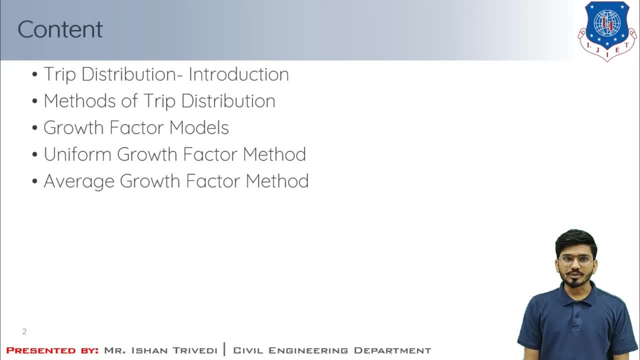 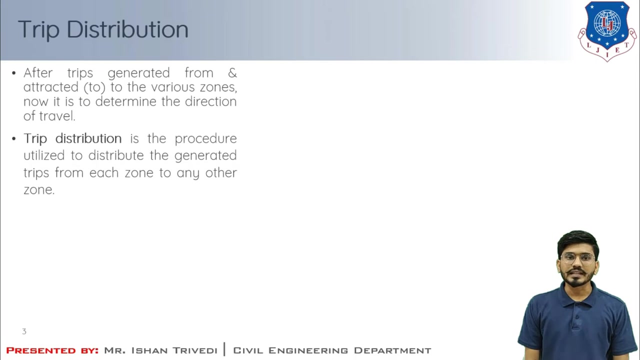 I am going to cover the trip distribution with its introduction, then methods of trip distribution. One of the trip distribution method is the growth factor models, in which in this session, I am going to cover the uniform and the average growth factor methods. So first we will understand what is trip distribution. After obtaining the trip estimation that the 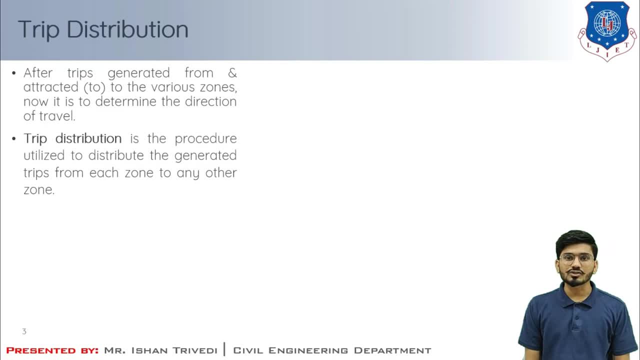 generated from zone and attracted to the various zone. it is necessary to determine the direction to travel. Here the number of trips generated in every zone of those study area has to be distributed to the various zone to which these trips are attracted. Here the trip distribution. 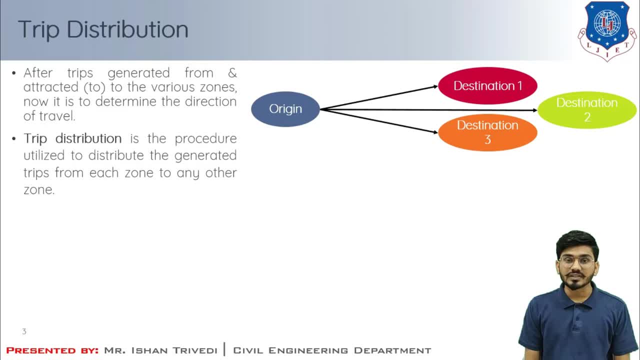 is the procedure utilized to distribute the generated trips from which- or you can say, from those zone to any other zone. In a simple example, in your house you have your working parents and, inclusive of you, there are three members, and three members are traveling to different zone. One is going for the study purpose and rest of the two are working in. 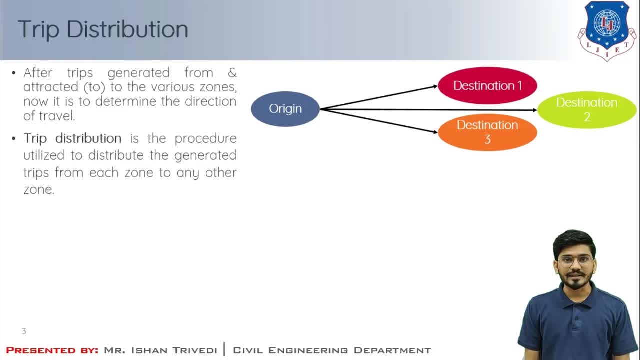 different zone. So here the origin remains same, but the distribution of various destination is been different and that's why the origin that we have calculated, that the number of trips are generated from X zone to Y zone, that I have, but how these trips are distributed among those zones and the areas, that we have to computed, and these will be done in this. 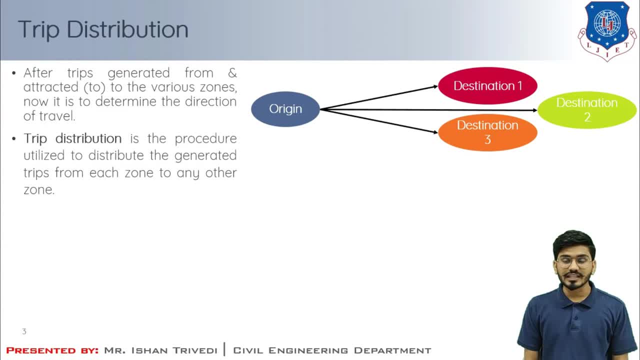 trip distribution, that whatever the trips are generated between the zones, how they are distributed, And this will be done in this trip distribution, In this trip distribution, we will compute the trip distribution matrix Here. the purpose of this trip distribution model is to distribute the zonal trip in order to predict the flow of trip, that is, Tij, from each production zone. 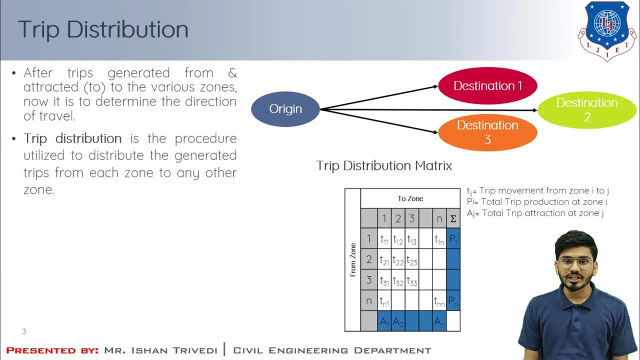 I to the each attraction zone J. You can see here Tij, For example, the flow of trip distribution matrix is like this: You are residing in the zone one and there are three zone, that is, zone one, two and three. If your mother is going for taking the vegetables then it is of interzonal. 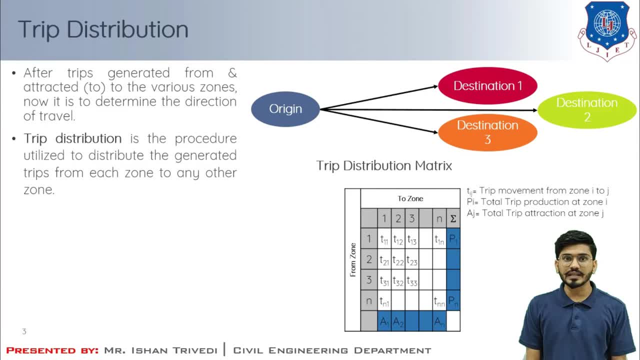 or within the zonal activity, that is, the trip is been started in the zone one and end with the zone one. If your father is working and if he is traveling from one zone to second number zone, then the trip is distributed Between T12. then, where T1 determines that they have started their journey from, you can. 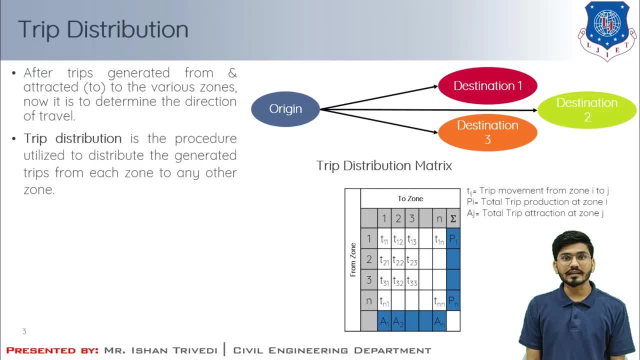 see here from zone. So it notes where the journey has been originated, where J is the destination of the trip and that is here. it is two because the father has traveled from zone one to two. So it is in terms of Tij. So it is in terms of Tij. 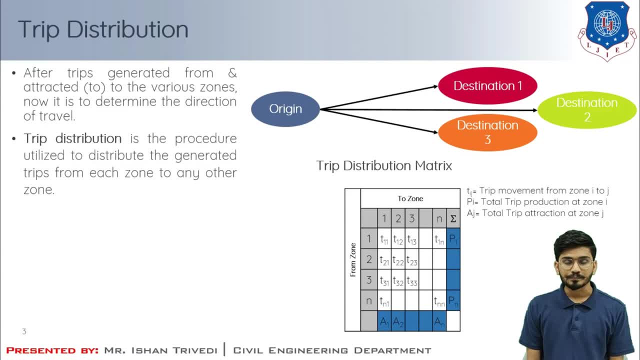 So it is in terms of Tij, It is T12.. You can see here, and if you travel from origin, that is zone one, to the college or the school, then it is the destination three in that other zone and that we call it Tij, and that is T13. 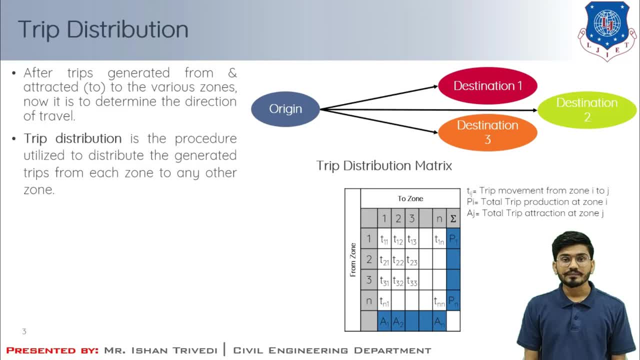 So this is how our trip has been distributed, and that number is nothing but the summation of all those trips that have originated from zone one And distributed in the zone one, two and three. so furthermore, I will discuss here the properties of those synthesized trip distribution matrix are described here- that I have elucidated there. 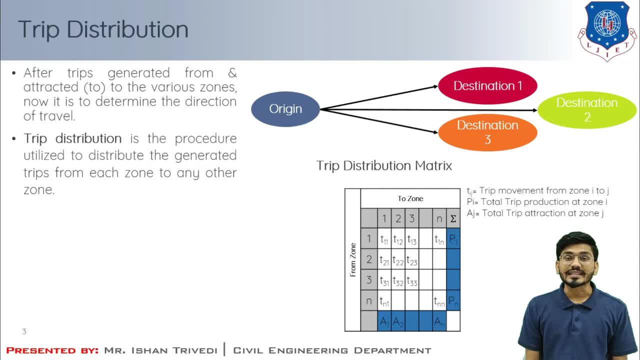 are n number of zones and n number of activities which are involved, means n number of destinations are there. As I told you, if there are three zones, then there are three types of activities within the zone, in zone two and zone three. then in this urban area, what I will get, I will get. 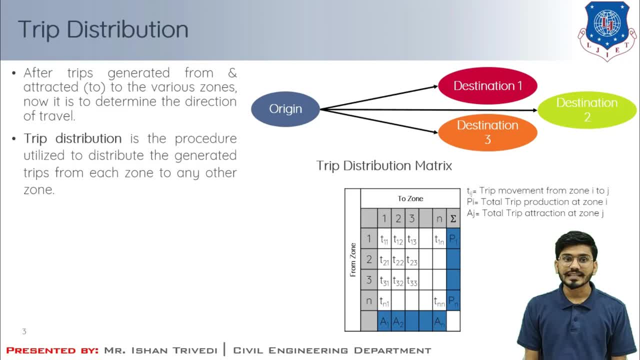 the matrix of n by n- and here it is n- square possible movement in that particular urban area. and any trip distribution matrix has to satisfy these two criteria. one I have already told you again I will tell you in the equation form, that is the summation of trip movement. 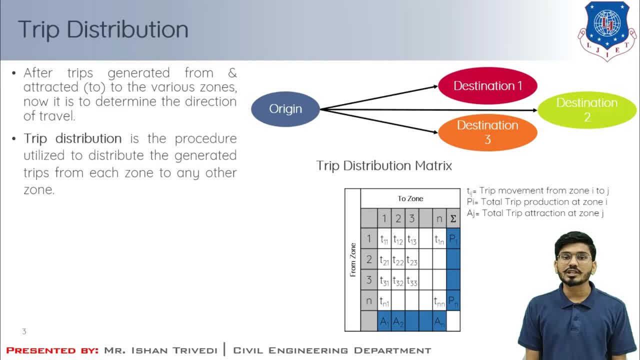 from zone I to J must be equal to the total trip produced from the zone I. So in zone I means where you are residing, your residential place is zone I and where you have distributed the destination, one destination, two and three: school or college, then workplace or any vegetable market, then thus our three trips are distributed where. here, how you will. 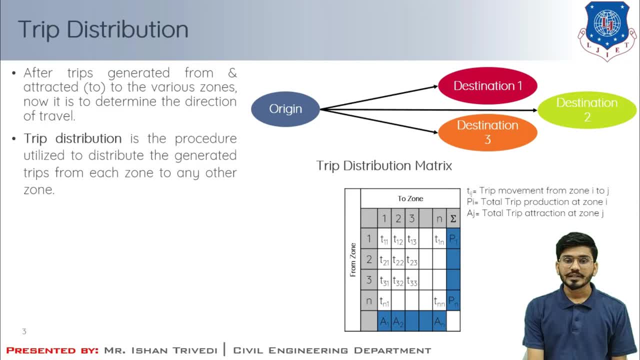 find this distribution of trips here. whatever the production of trips has been done, it is find out here in terms of these entries, and that is our row entries. here you can see the origin zone from zone and the destination zone. here it is written now: our from zone. 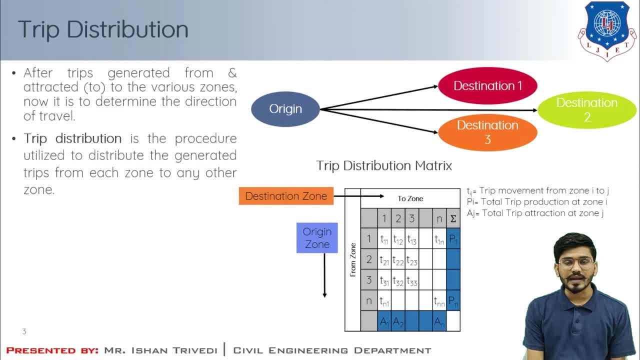 that is our origin zone, that we have T I value. I value denotes our origin and J value denotes our destination. so I have started my journey from zone one and it has finished in zone one. then it is called T11 value. here you can see T11 value. here it is T11 value. then if I start my journey from zone one and if it, 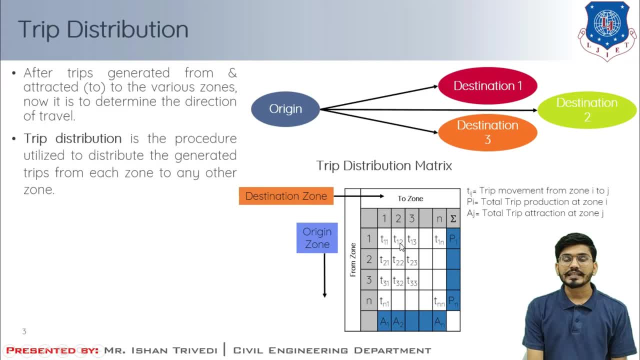 is ended in zone two, then it is called T12 value. similarly, if I start my journey, just wait for a while- If I start my journey from zone two and if it ends at zone three, then it is called T23 where from the zone where I have started my journey, it is called I. that is called production. 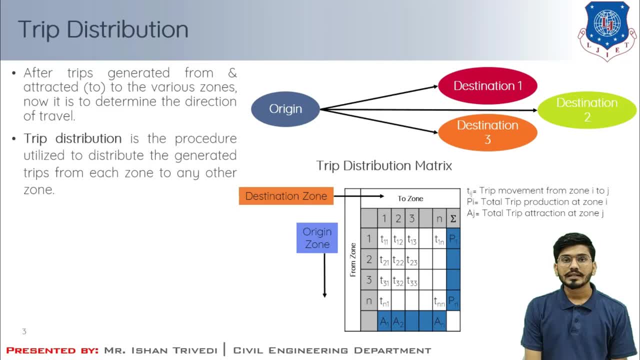 and where I am ending my journey. that is called attraction and it is called J for production. we denotes it by P and for attraction we denote it by A- that we have learned from the trip generation model. So here, all those row values are nothing but our P. I value that. I am telling you that. 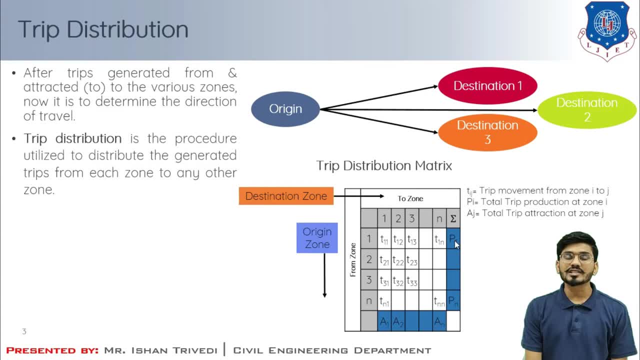 summation of all the trip moment from zone I to J must be equal to the trip production of that zone I. and if I make the summation of all those trip it is nothing but my P1 value for zone one. Similarly, if the summation of those trip moment from zone I to J must be equal to the total, 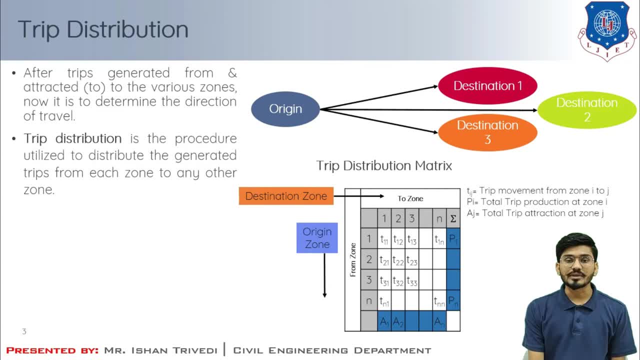 trip attraction to zone J, Where all those trip moments from zone I to J must be equal to the total trip attraction to zone J. All the summation of column will be done. that from zone one to one here the my attraction, and I will make the summation of these values, that is, our column value, will give me the 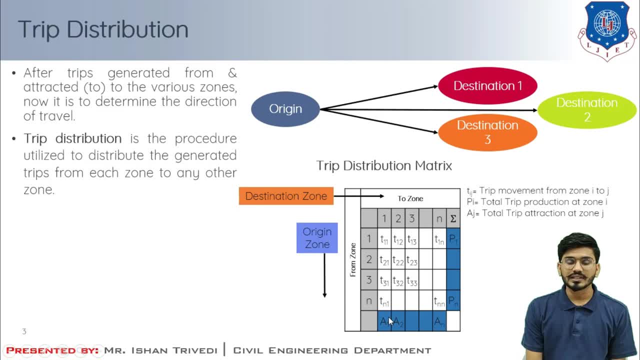 attraction value. So here you need to understand that is: Tij is the trip moment from zone I to zone J, then Pi denotes the total trip production from zone I and Aj denotes the total trip attraction to zone J. Now understand the trip distribution function, how it is functioning here: zonal, socio-economic. 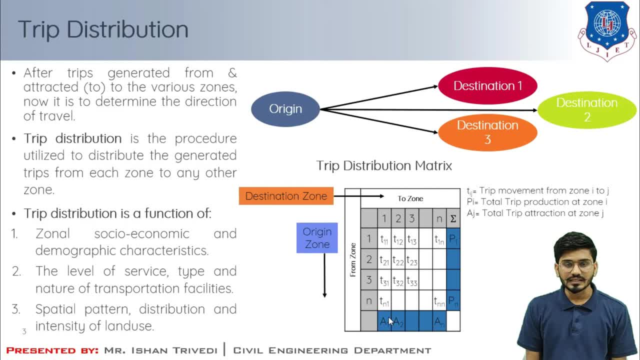 and demographic characteristics has been captured, then the level of service, the type and the nature of transportation facilities need to be checked and, at last, spatial pattern of those urban area and how those distributed Various land use and how the intensity of land use is been distributed among those spatial. 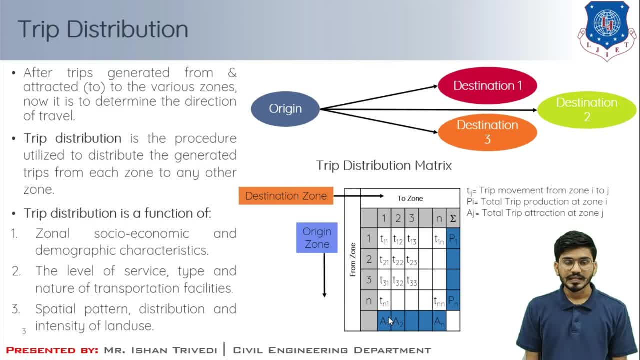 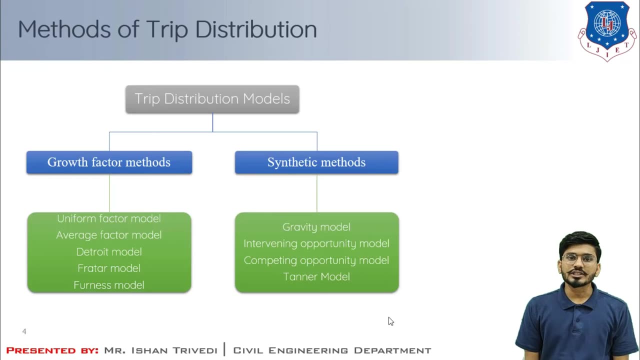 pattern or form of the urban structure and based on that, my trip distribution are dependent. So now understand the methods of trip distribution. there are several approaches to the trip distribution and these are broadly classified in two categories, That is, growth factor, more methods and synthetic methods. 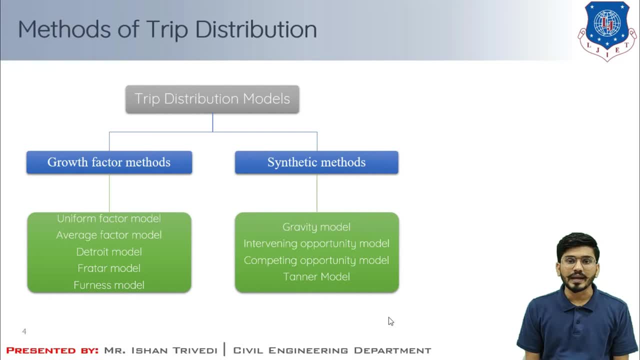 These methods are based on the principle that the trip moment increases with increase in the attractions and of that particular type of travel and it decreases with the increasing in the impedance to travel. here the trip distribution models, in particularly growth factor models, are classified as a uniform factor model, then average factor model, Detroit model. 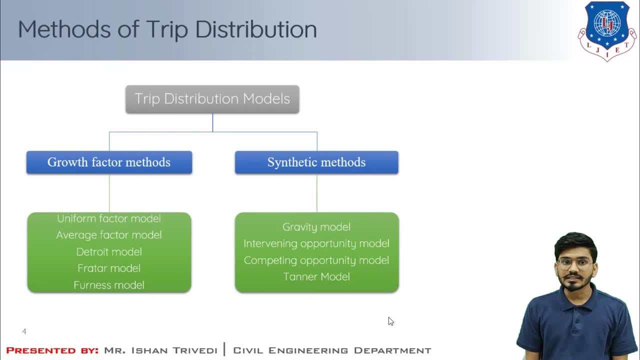 Frater model and the furnace model and the synthetic models are of gravity model, which is one of the important model, then intervening opportunity model, competing opportunity model and Tanner model. So we will study all these models in our next succession and next upcoming lectures. So first we will study 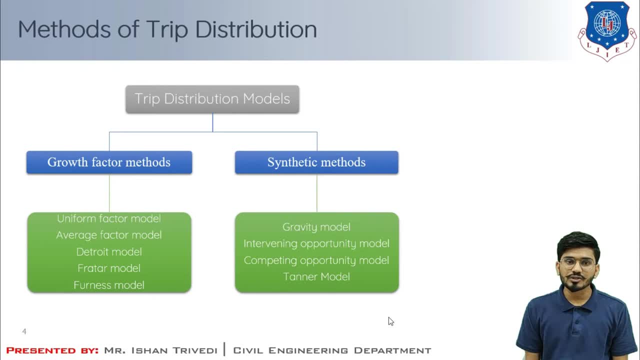 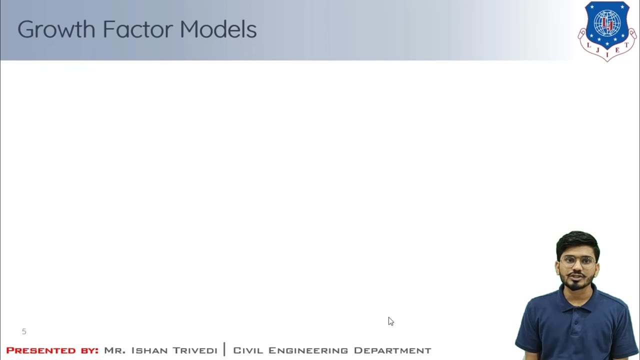 First we will start with our trip distribution model and that is the growth factor models. in growth factor models, As I told you, there are total five number of models, that is, uniform factor model, average factor model, Detroit fact, Detroit model, Frater model and furnace model. in the growth factor model, the base year trip. 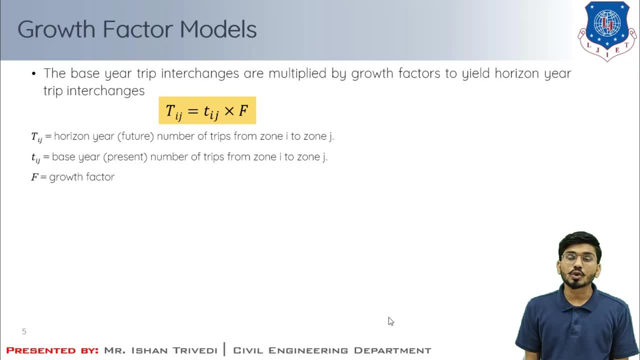 interchanges are multiplied by the growth factor that we are calculating, and it is the yield of horizon year trip interchanges. here it is given in this form. that is the general equation. that is capital. Tij is equal to Tij into F. here F denotes the growth factor. 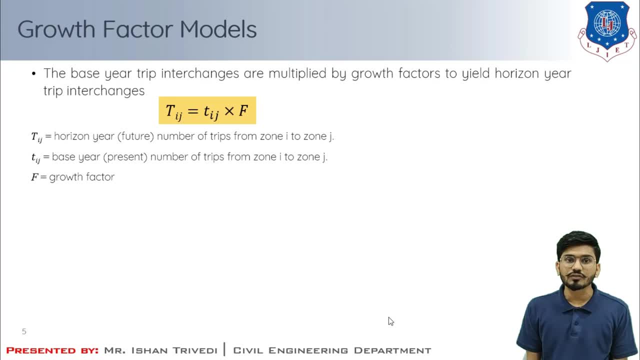 and capital. Tij is the horizon or you can say futuristic number of trips that are going to be produced between zone I and zone B, Zone I and zone J, and small tij denotes the present value of those trips which are already generated from zone I to J. that is of present value, and capital denotes the futuristic value. 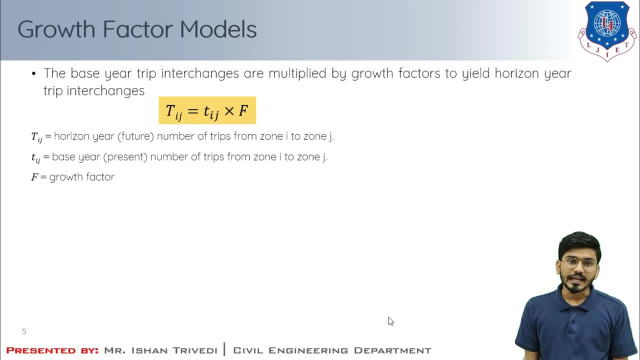 and if I want to calculate the future value, what I do, I will calculate the growth factor. it is a general term, general equation for all these model. Here the value F will be change based on the model. so if I am talking about uniform factor model, the standard equation will remain same, but there may be change in the growth factor. 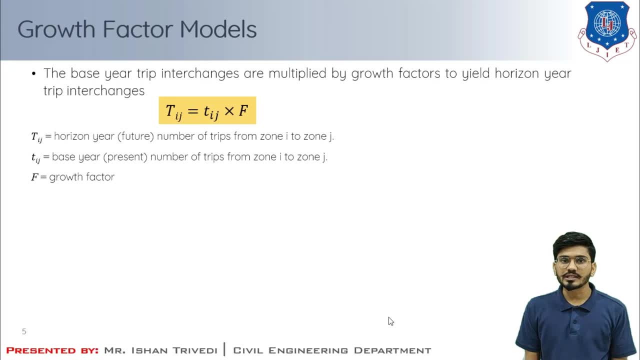 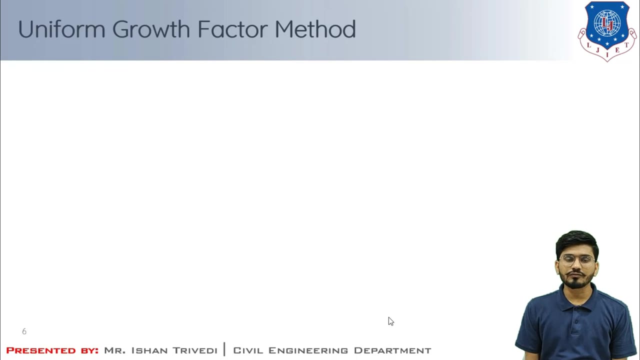 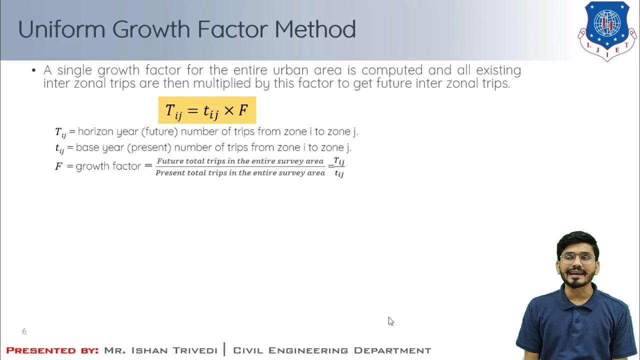 model and the calculation method. but the standard equation will remain same that in present trip. if I multiply the growth factor I will get the futuristic trips. if I am talking about the uniform factor model or uniform growth factor model, then in this method a single growth factor for the entire urban area is computed, means for all the zones I will compute only. 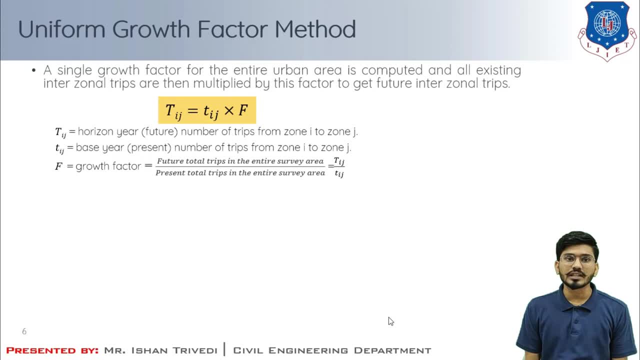 one growth factor and all existing interzonal trips are then multiplied by this factor only and we will get the future interzonal trips. here you can see the equation that is: Tij is equal to small. tij into F, Where capital Tij denotes the future number of trips from zone I to zone J, then small. 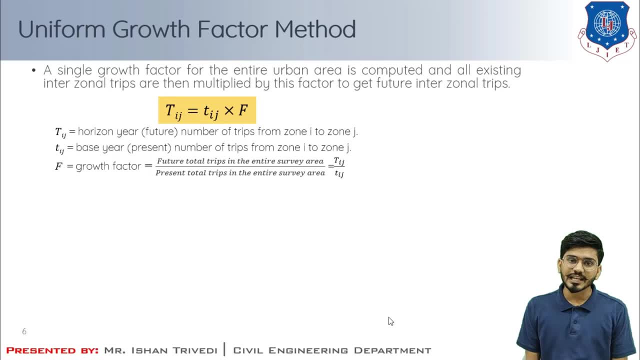 tij denotes the base year, means present number of trips from zone I to J and here F denotes the growth factor and that is the future total trip in the entire survey area. capital Tij upon the present total trip in the entire survey area and that is small tij and based 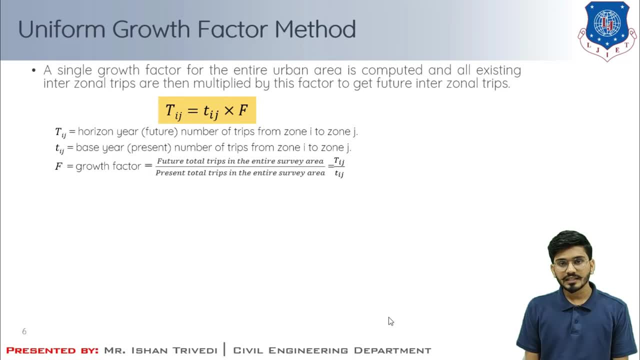 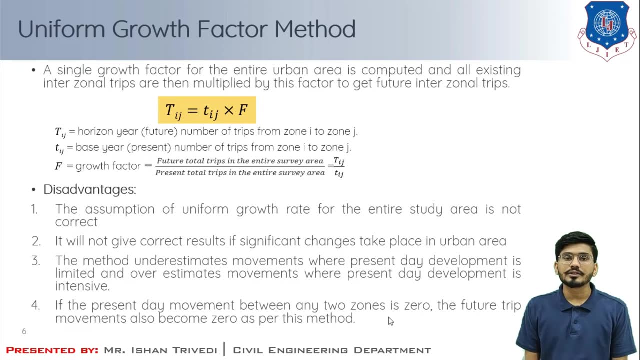 on that. I will calculate the growth factor here. there are some disadvantages of this uniform growth factor method. the assumption has been taken that the uniform growth rate will apply to entire study area, which is not correct, and because of that each zone will have its own growth rate and we have to calculate the individual growth rate of inner interzonal. 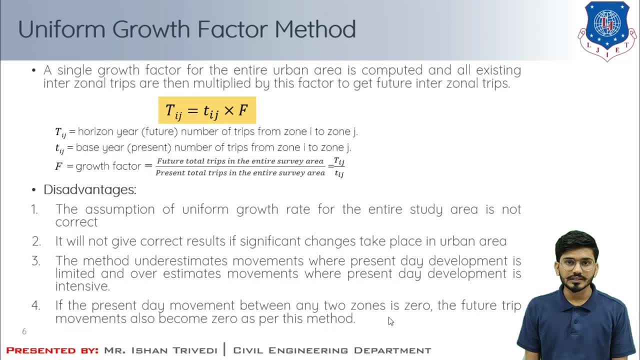 activities that will further study in upcoming months, Then it will not give you the correct result if the significant changes that has taken place in the urban area, like concentration of population, if the industries would arise and there are other commercial activities which are happening, or in future if they are. 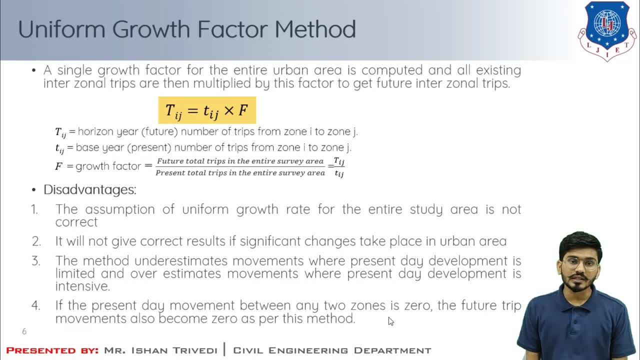 if there is any change, then it does not give us a correct. well then, the method which underestimate the moments where the present day development is in progress And overestimate where the moments where the present day movements or development is intensive means when there is a lesser movement or limited development, there may be chances that there 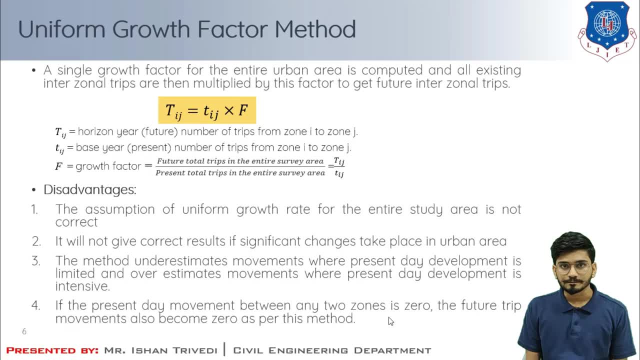 will be lesser movement and that assumption has been taken. if there is an intensive development is there, then the value will be overemphasized and overestimation has been done. if the present day movement between any two zone is zero, then it has been assumed that in future also. 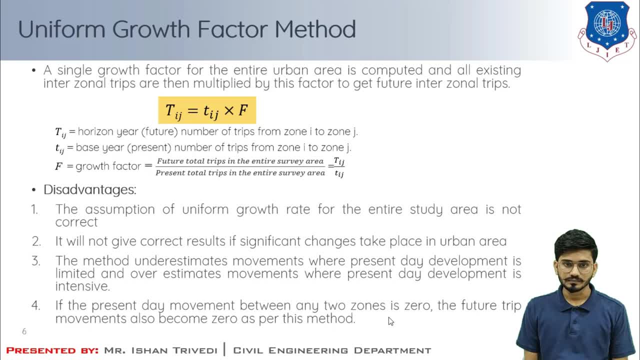 this value will remain zero, and this may rarely be in case of the reality. in any zone, there may not be a zero trip or any interchanges in future if the present situation is that there is no interconnection of any trip that has been generated from one zone to another. 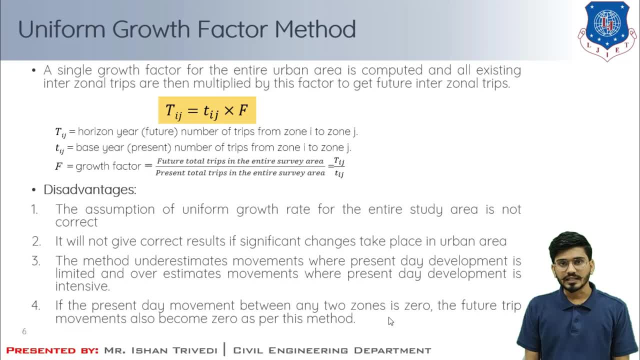 zone, then it is okay. in present condition this would have happened. but in case of future, you cannot say that in future there will be no trips at all. so here this model or this method fails. next is the average growth factor method that we will study. so in average growth, 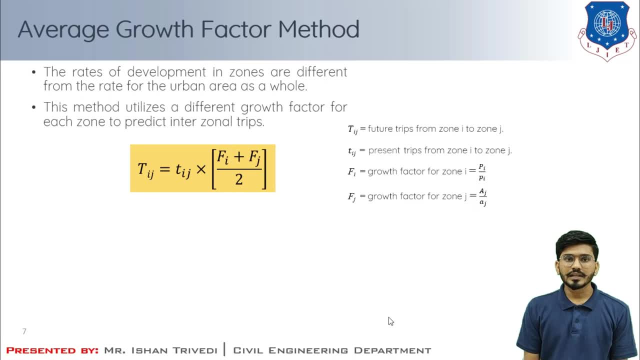 factor method. here I am going to take the account of fact that the rate of growth is the rate of the development in zone are normally different from the rate of what we have computed for the urban areas whole. so here what I will compute. I will compute the average value of 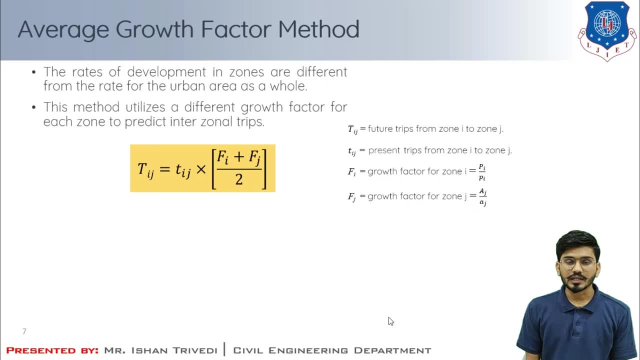 those growth factors in what we have computed from the production side and what we have computed from the attraction side. so in this method it is utilized a different growth factor for each zone to predict the interchanges. Here the equation has been given, that is, capital Tij is equal to small tij into fi plus fj upon. 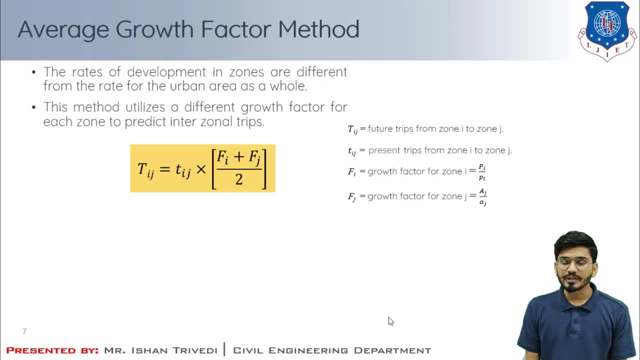 2, where tij is the futuristic trip between zone i to j, then small tij denotes the present trip between i to j, then fi denotes the growth factor for zone i and that is the futuristic production pi upon small pi that is of present value.